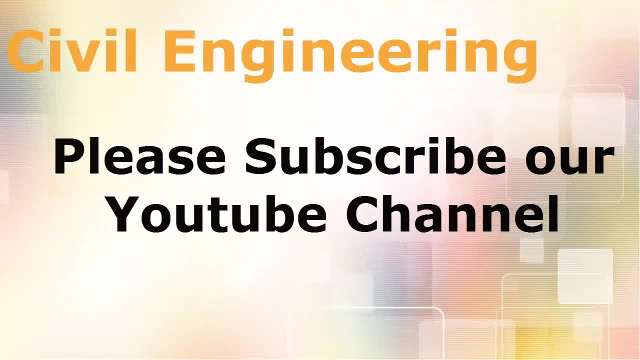 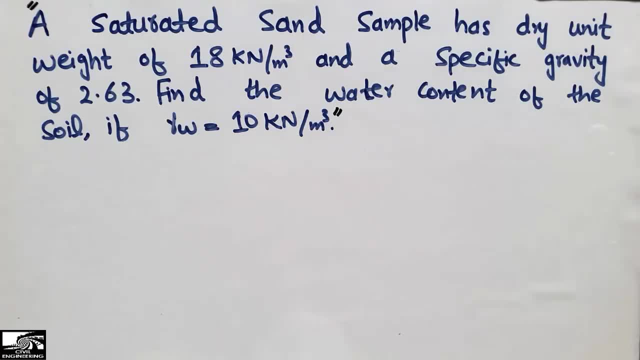 Hello guys, welcome back to the C1 Engineering YouTube channel. Please subscribe our channel for daily C1 Engineering videos. Today our lecture is about the soil mechanics and we are interested to find the numerical in the soil mechanics. So this is the problem given to us and we want to find the unknown parameter in it. 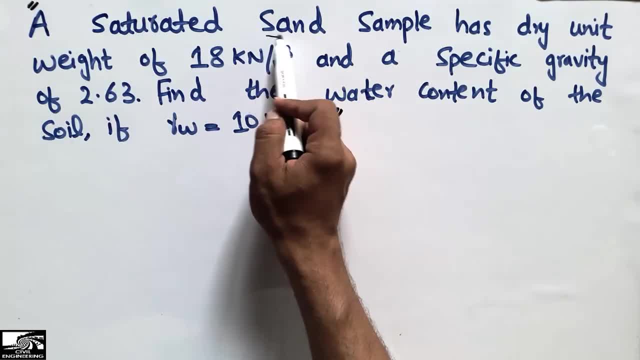 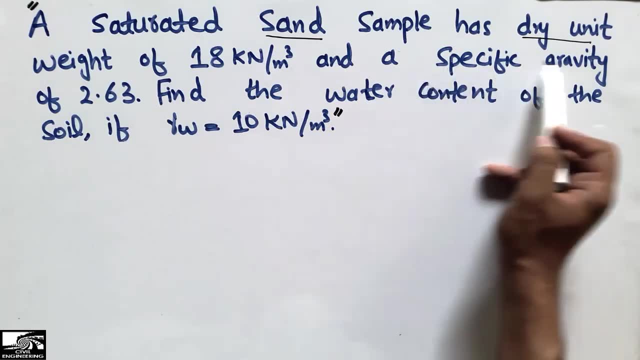 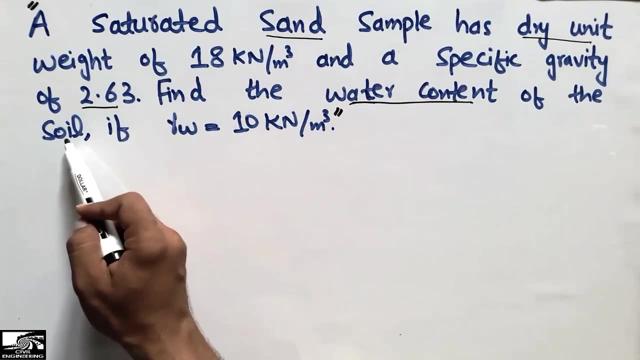 So the problem states that a saturated sand sample right. saturated sand sample has a dry unit weight of 18 kN per cubic meter and this sand has a specific gravity of 2.63.. So find the water content right. we will find the water content of the soil of this sand sample right. 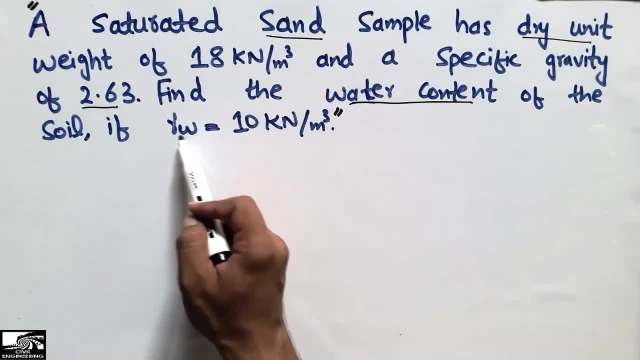 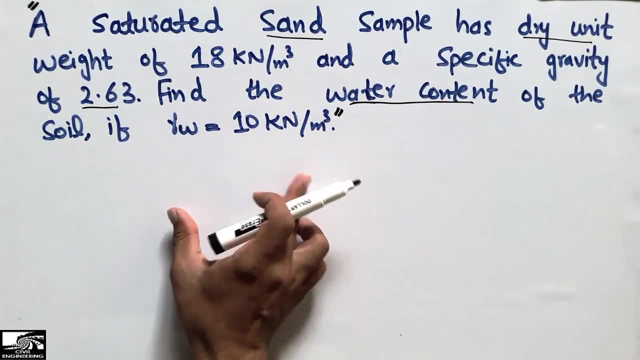 if the gamma w, the unit weight of water, is 10 kN per cubic meter. So there are some parameters given to us, Like the sand sample has the dry unit weight and it has a specific gravity and the water unit weight and we want to find the water content, that how much water content is present in this sample? sand sample. 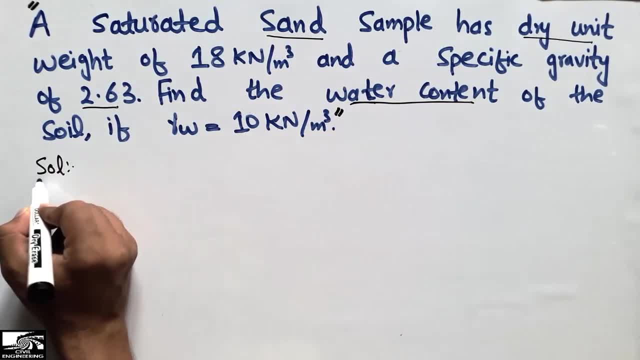 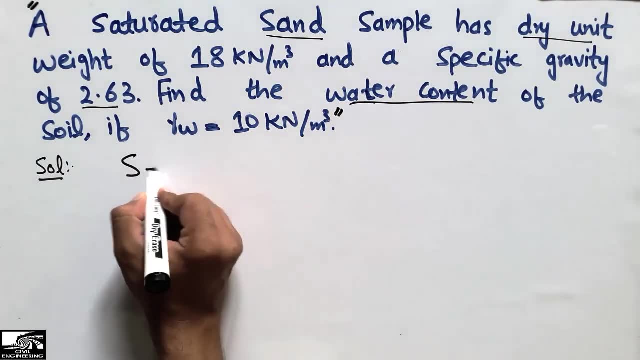 So to start the solution of this problem, as we know that it is given that a saturated sand sample, right, so a saturated sand sample. so it means that the degree of saturation of this sand sample is equal to the 1. It has a dry unit weight of 18.. 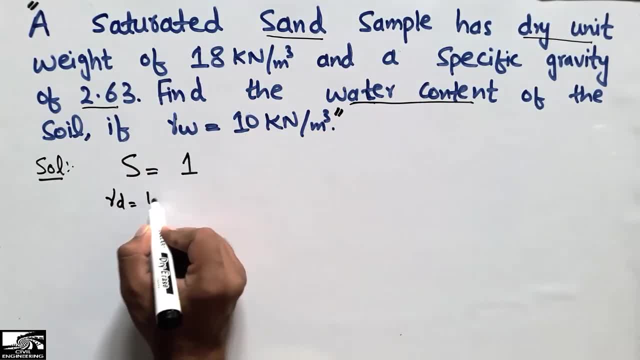 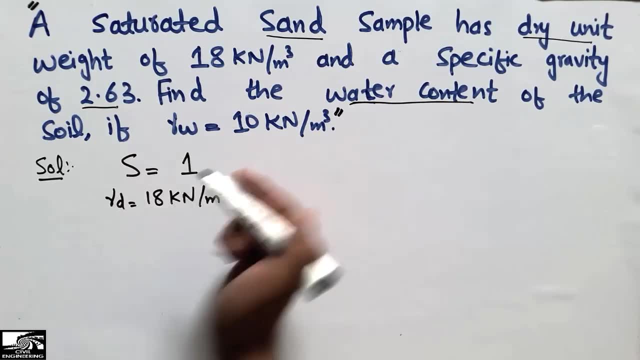 So we can find the dry unit weight of 18.. So we can write it that it has a dry unit weight of 18 kN per cubic meter. right, It is the unit weight. the dry unit weight of this sample is 18.. 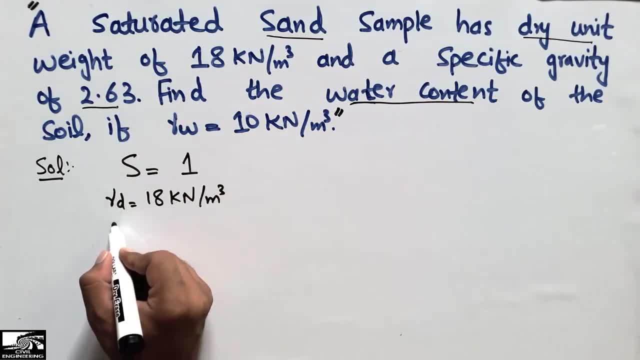 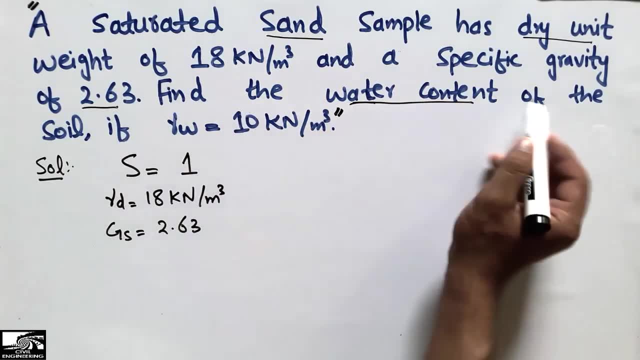 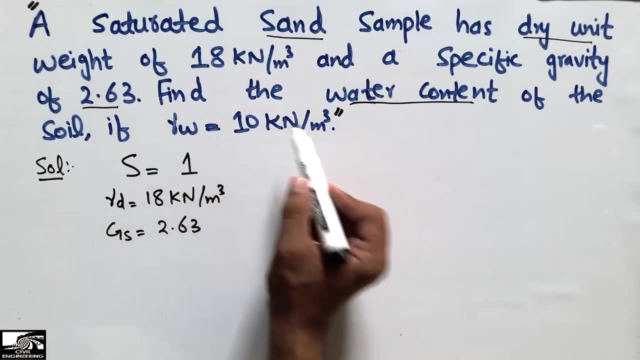 Now, and it has a specific gravity of 2.63.. So I can also mention that the specific gravity of this sand sample is 2.63. And find the water content of this sample, sand sample and it has the if the gamma water, if the gamma w is 10 kN. 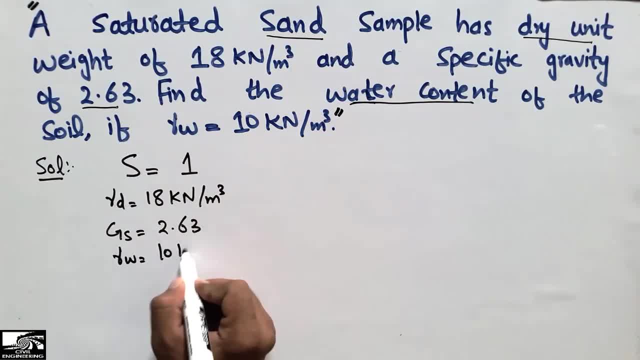 If the gamma w is 10 kN per cubic meter, I want to find the water content. that how much water content is present in this sand sample. So to start the solution, I have a simple formula to find the water content right. 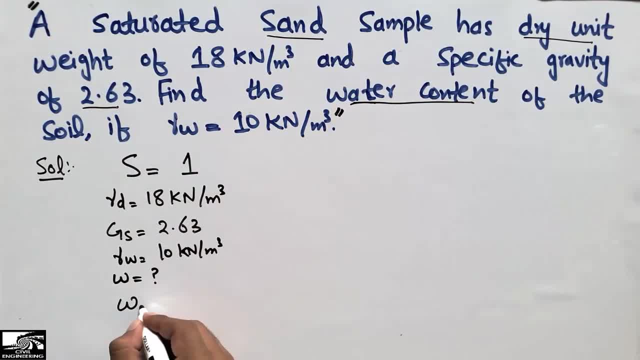 So I will use this formula: w into g is water content into specific gravity is equal to the s into e. We will search different formulas to find the unknown parameters, Like in this case. I want to use this formula from the sand mechanics, from the different types of formula. 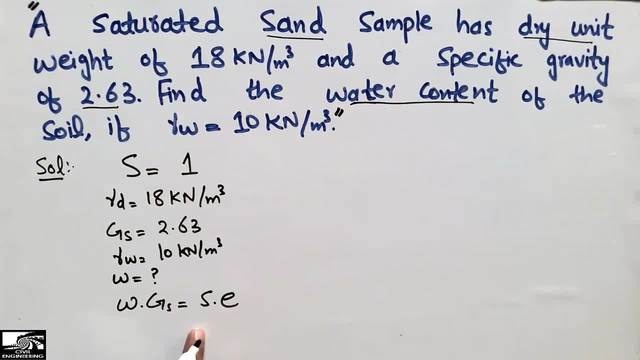 Why? Because there are some unknown parameters to us, so it will be easy to find the unknown. I will also upload a separate video on the sand mechanics formulas. Please check the video on the link: I have given the link in the description. 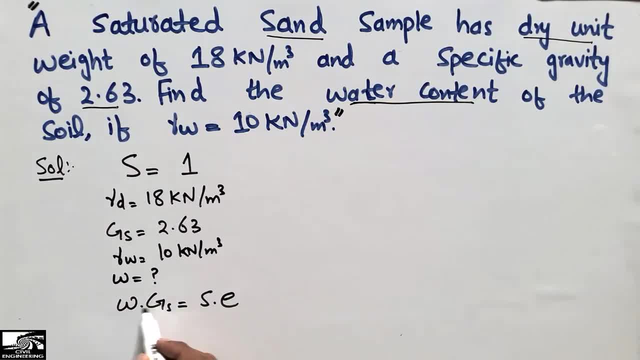 So, by using this formula, the water content into specific gravity is equal to e. Specific gravity is equal to the degree of situation and to the w ratio. But here again we know that we will find the water content right. Specific gravity is known to us, which is 2.63.. 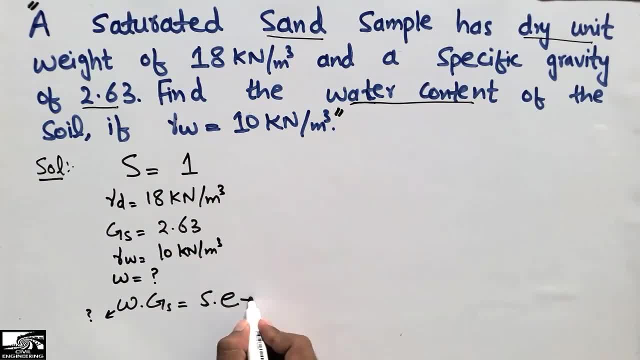 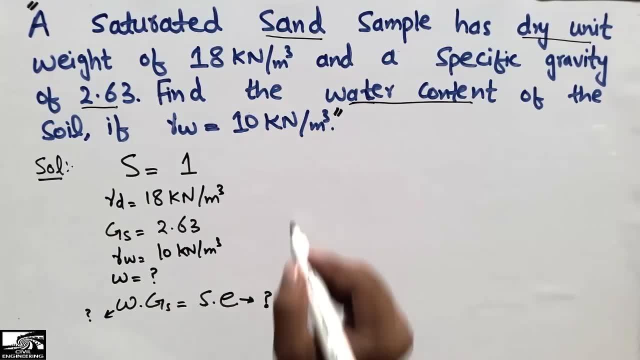 The degree of situation is one which is known to us. but this w ratio is also unknown to us. So what will we do? First, we will find the w ratio. So we can find the w ratio by another formula which states that the gamma d, the dry unit, weight formula. 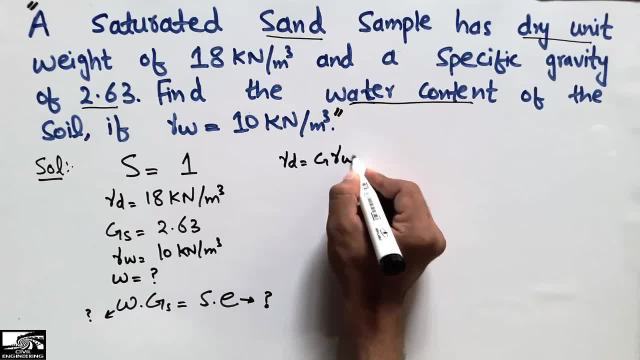 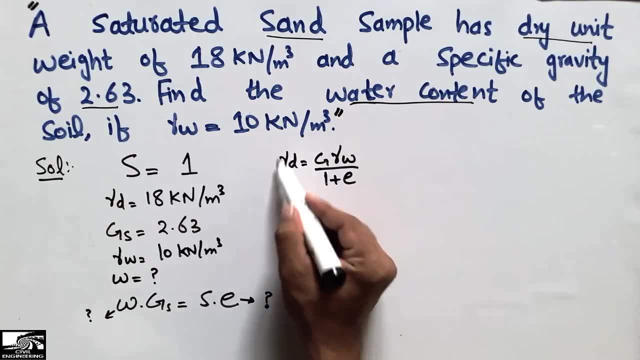 I have given a different type of formula. I have given a different type of formula for using the sand mechanics. So check this video on the link please. 1 plus e. So this is the dry unit weight formula. So to find the e right, I will transfer this side portion into this side. 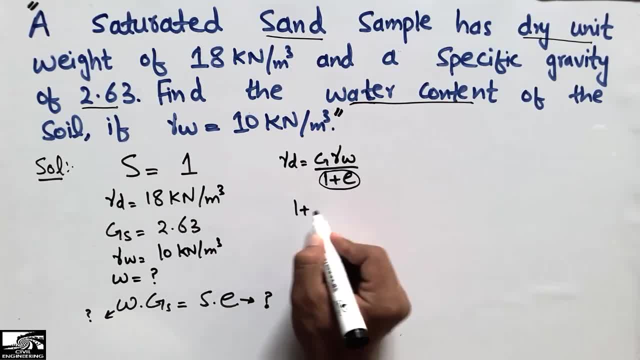 And I will transfer this gamma d into denominator. So it will be simple: 1 plus e is equal to e. It's simple mathematics. Gamma d, the above one, is the same. Now gamma d will be, comes out into denominator. 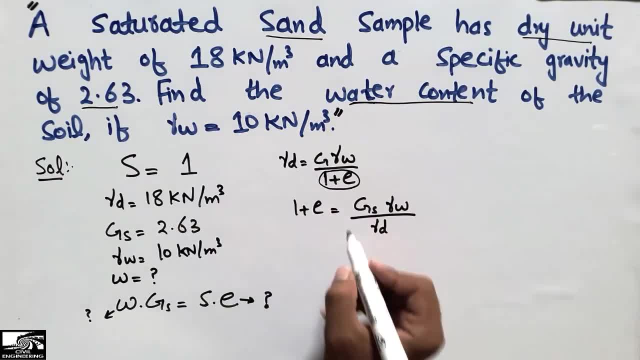 So it's very simple, just crossing these two elements. So now 1 plus e, right, So I can know that the 1, so I can write the e is equal to the gs specific gravity into the unit weight of the water, into the gamma d, into minus 1,, right? 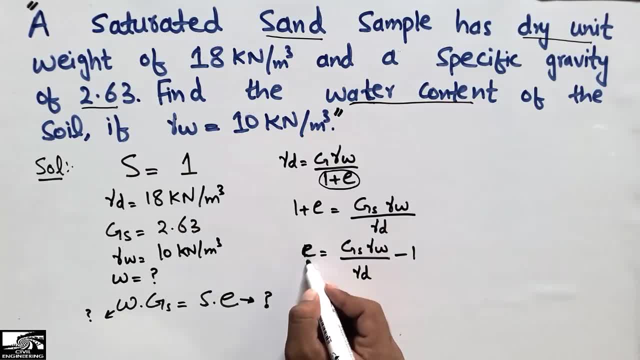 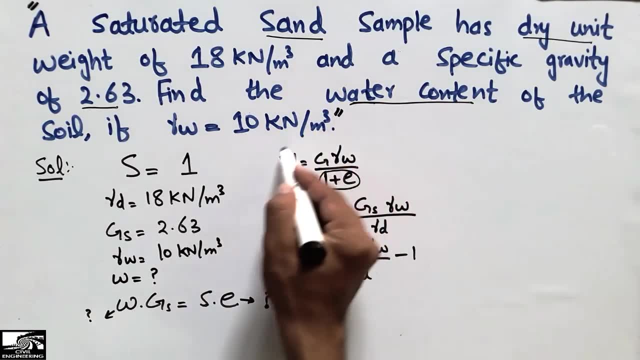 I shift this one here into this, So now I will find the w ratio. So then I will put this w ratio into this formula, so to get the water content. Now I use this formula to find the w ratio because we know that the dry unit weight of the soil is known to us. 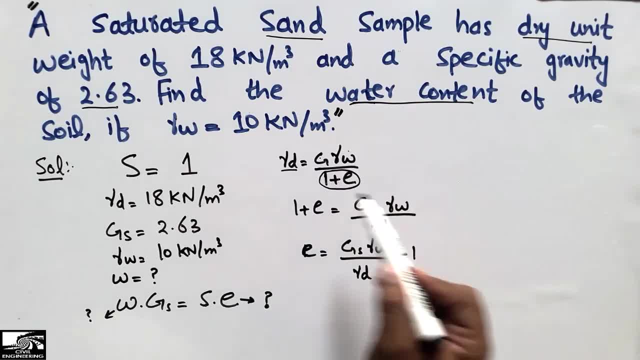 the specific gravity is known to us and the gamma w is known to us. That's why I use this formula. Otherwise I should switch to the other formula. So in this case all other are known to us. g is 2.63, gs you can see here, and the gamma w is 10 here. 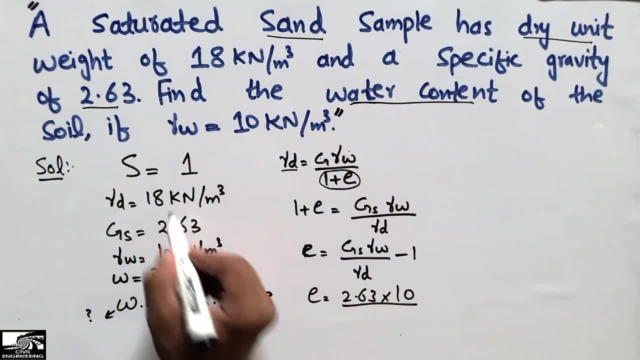 You can also see: gamma d is the dry unit weight, which is 18 here and minus 1.. So I'm just by calculating this value, I get the answer of 0.46.. So the w ratio comes out to be 0.46, right? 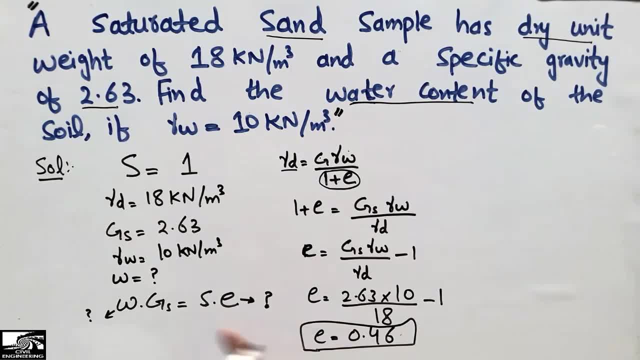 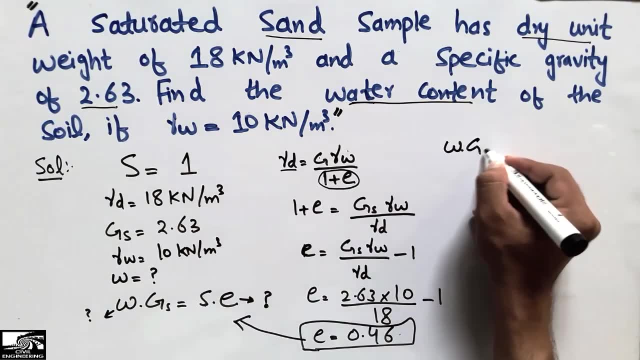 So now I will put this w ratio into this equation so I will get my water content. So by putting this value here into this equation, so w into gs is equal to this degree of situation into w ratio. So by w, by transferring this value here into the other portion, 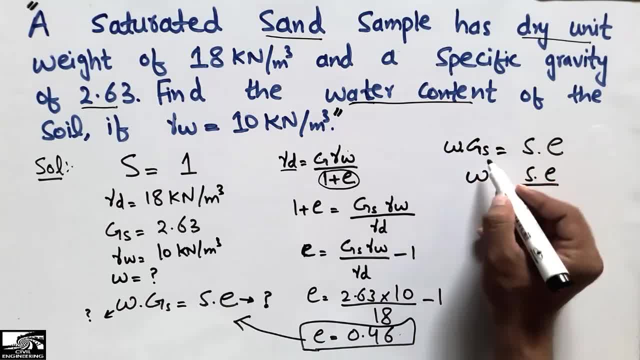 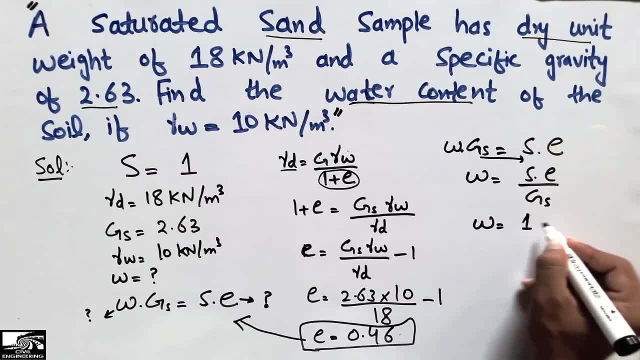 so it will come out into division, right. It is a multiplication here, so this portion will come out into division, so it will be gs, right. So now the water content is equal to the degree of situation. is 1 of this sand sample. 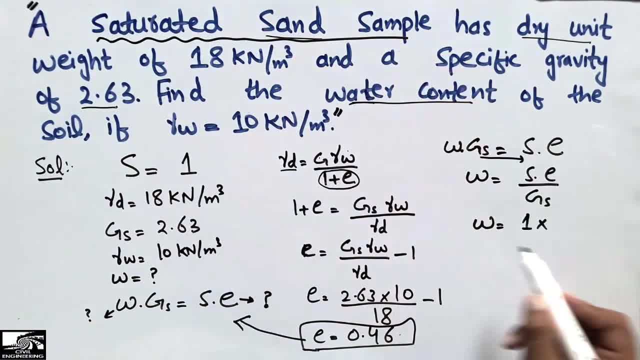 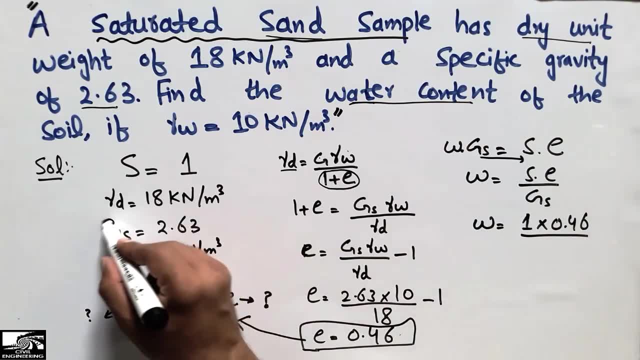 because it is still. it is a saturated sand sample, So the degree of situation will be 1, e is 0.46, as I found out here, and the gs of this soil sample is sand sample is gs 2.63, right. 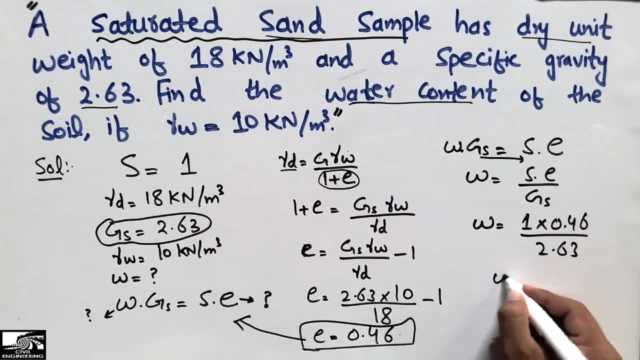 2.63.. So by dividing these parameters I get my answer of 0.17,. right Now, by multiplying it with the hundred, I will get my water content in terms of the percentage. so it comes out to be 17%. 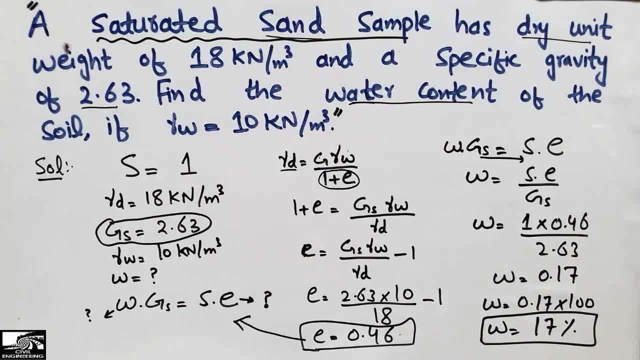 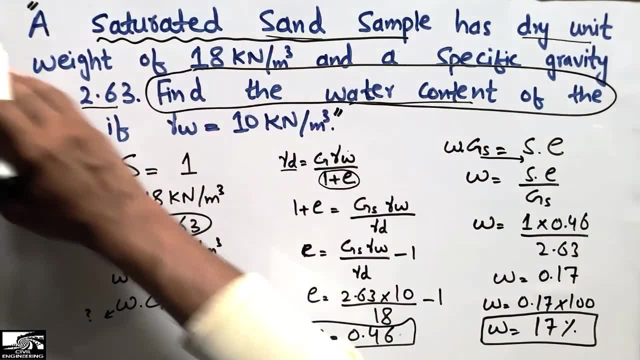 So my water content of this sand sample is 17%. I found out that the water content in this sand sample is 17% If the saturated soil sand sample is a dry unit weight of 18,, specific gravity 2.63, and the gamma used of the water here is 10,. 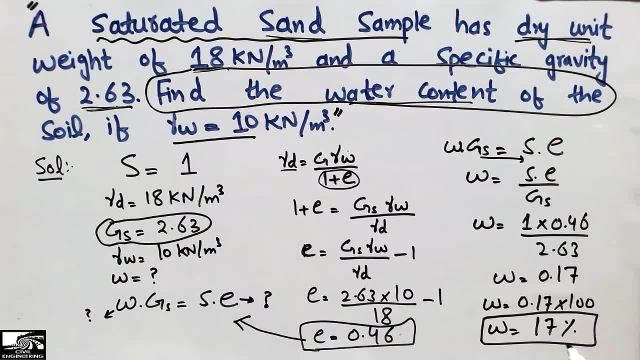 so then my sand is is a water content of 17%. Hope you guys understand. This is the formulas- different formulas used in the sand mechanics. So I used the two formulas, this one and this formula. right, So you can use the different formulas according to your unknown parameters, right?